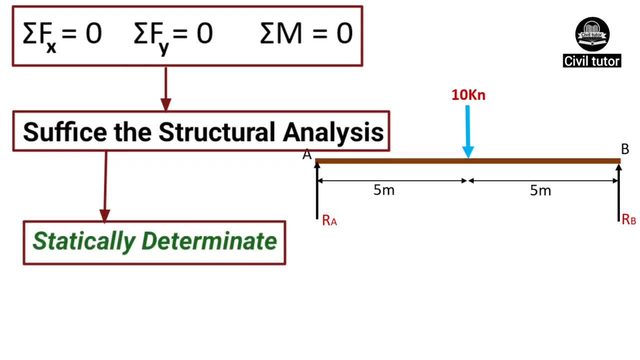 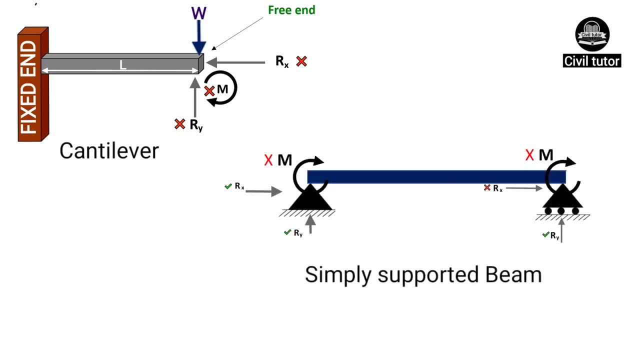 categorized as a statically determinate structure. In simple words, for a determinate structure, the number of unknowns or reactions is equal to the number of equilibrium conditions. For example, cantilever beams, simply supported beams with one end hinged and another end on. 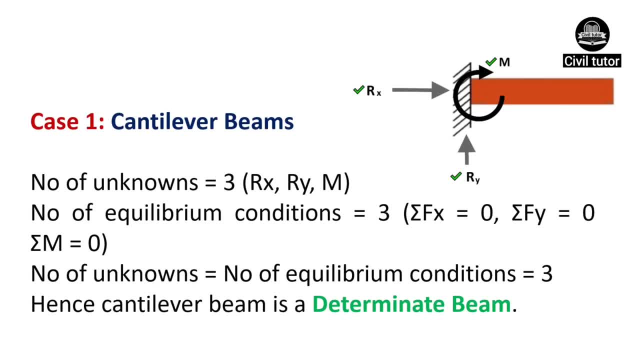 roller support. If we talk about cantilever beams, it has two ends, ie fixed end and free end. The fixed end develops 3D types of reactions, ie vertical reaction, horizontal reaction and moment reaction. The number of unknowns for cantilever beams will be equal to 3 ie support reaction Rx. 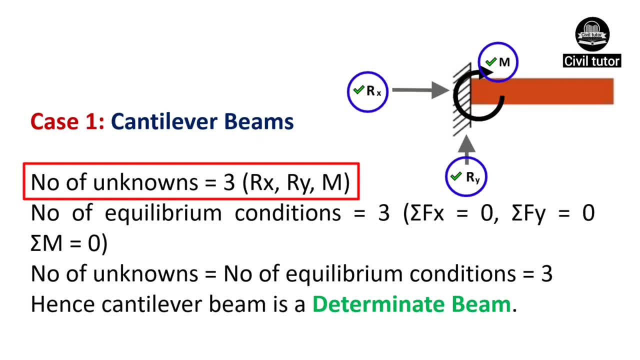 Ry and moment M, Number of equilibrium conditions is also equal to 3.. So the number of unknowns for cantilever beam will be equal to number of equilibrium conditions, which is 3.. Hence cantilever beam is a determinate beam. 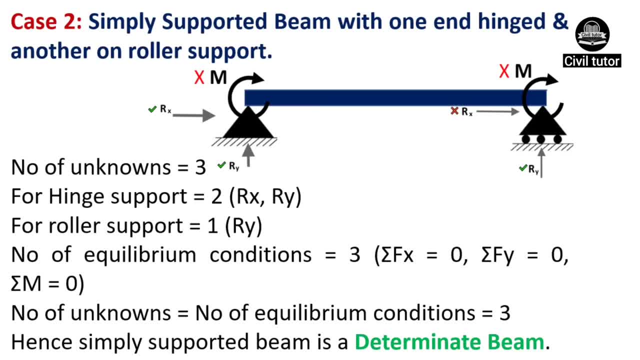 If we talk about simply supported beam with one end hinged and another end on roller support, it has three number of unknowns: Two for hinge support and one for roller support. For hinge support, it will have two reactions: ie, Rx and Ry. 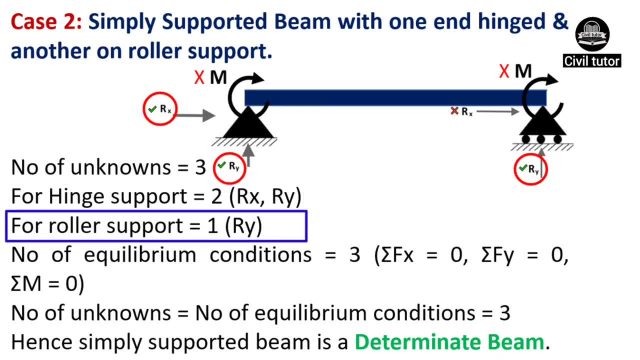 And for roller support it will have only one reaction, ie Ry. The number of equilibrium conditions is 3.. So the number of unknowns for simply supported beam will be equal to number of equilibrium conditions, ie 3.. Hence, simply supported beam is a determinate. 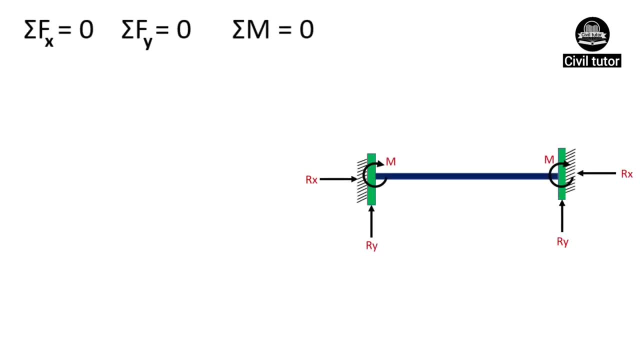 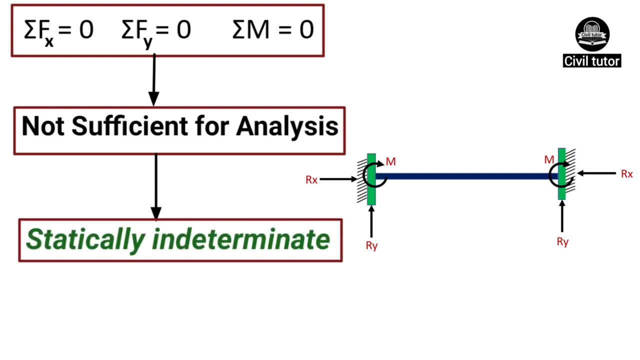 beam. On the other hand, if the equations of the static equilibrium do not suffice the analysis of a structure, the structure would be categorized as a statically indeterminate structure. In simple words, if the number of unknowns in a structure exceeds the number of equilibrium. 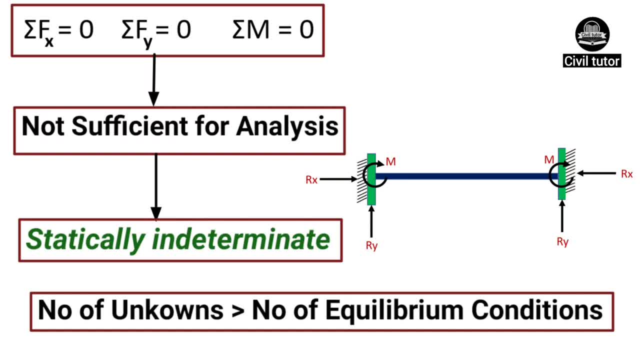 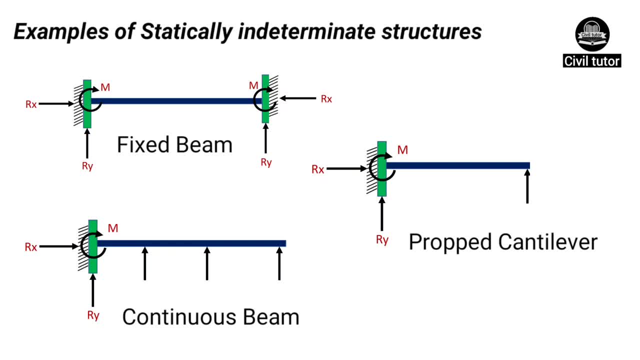 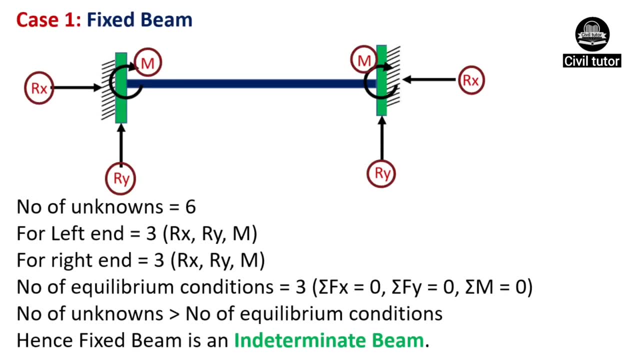 conditions, the structure is categorized as an indeterminate structure. Examples of statically indeterminate structures include fixed beams, continuous beams and proper cantilevers. If we talk about fixed beams, it will have six number of unknowns. For left-hand support, it will have three reactions: ie, Rx, Ry and M.